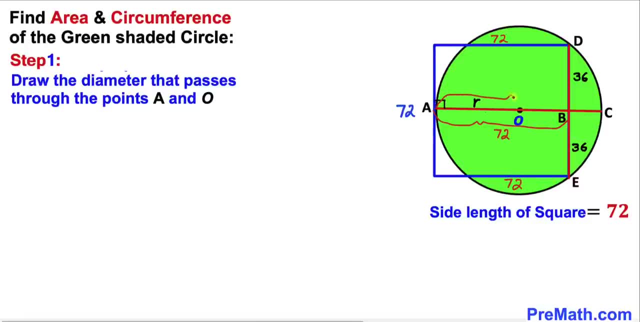 72.. We also know that this whole diameter is going to be 2 times the radius r, so therefore this distance b- c is going to be 2r minus 72.. Let me go and write down: 2r minus 72. and now we can see that we got these two chords, a c and d e, and they are: 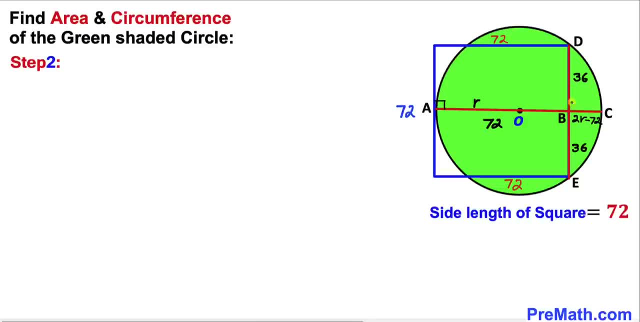 intersecting each other at point b. so therefore, we are going to recall intersecting this integral and in this example, we are going to recall intersecting the chords theorem. if two chords intersecting in a circle, then the product of the measures of the segments of the chords are equal, as you can see in this diagram. in other words, this a times b is going to: 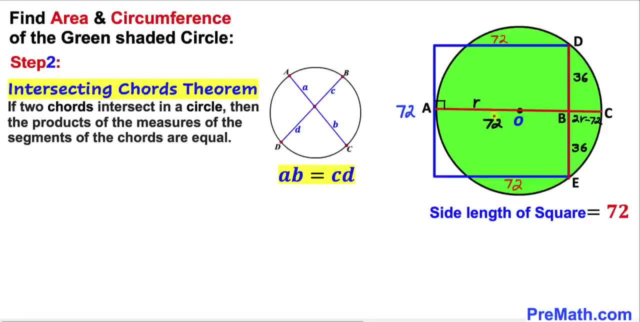 be c times d, as you can see over here. Now we can see: in our case our segments are singly and second. they are intersecting each other: 72 and this one is 2r minus 72. we are going to multiply them out. likewise, we got other segments. 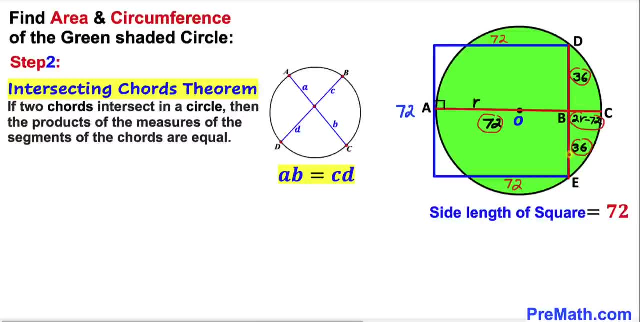 36 and 36. we are going to multiply them out as well. therefore, let me go ahead and write down: 72 times 2r minus 72, equal to 36 times 36. now let's go ahead and distribute this 72 that is going to. 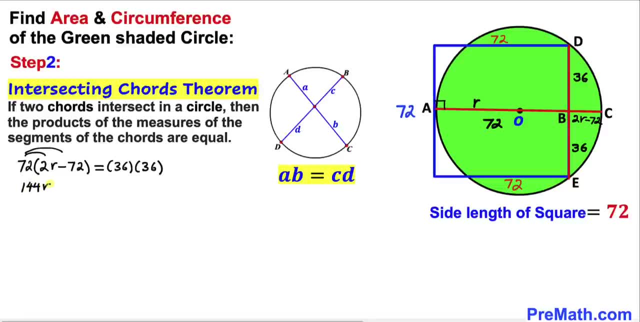 give us 144r minus. when we multiply 72 times 72, that is going to give us 51, 84 equals to 1296 on the right hand side. now let's go ahead and move this 5184 on the right hand side, so we are going to have 144r equals to 1296 plus 5184. let's go ahead and divide. 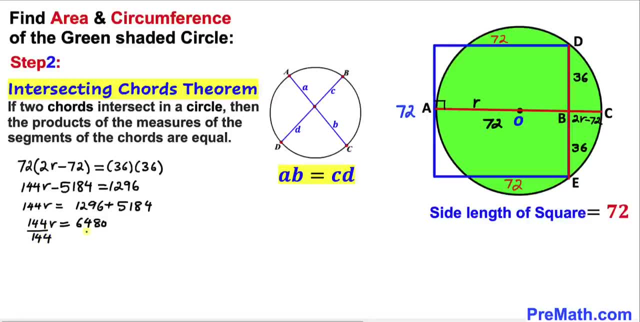 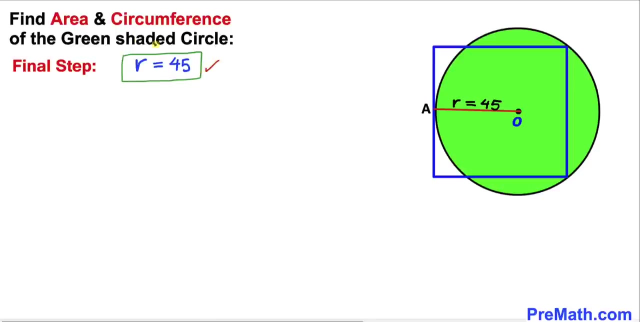 both side by 144, twice isolate r. so this 144 and 144 is gone. so our radius r turns out to be 45 units. and here's our final step. we already figured out our radius 45 units, and now we are going to calculate the area of this green circle. first and now let's recall the area of a circle: formula area. 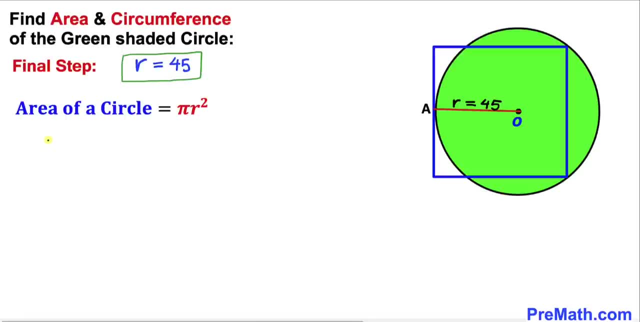 equals to pi r square. let's go ahead and fill in the blanks. so the area of this green circle is going to be pi times r, in our case is 45 whole square, and if we square that thing, that is going to give us 20, 25 pi. we know that pi is approximately equal to 3.14 if we plug it in over here. so our area is: 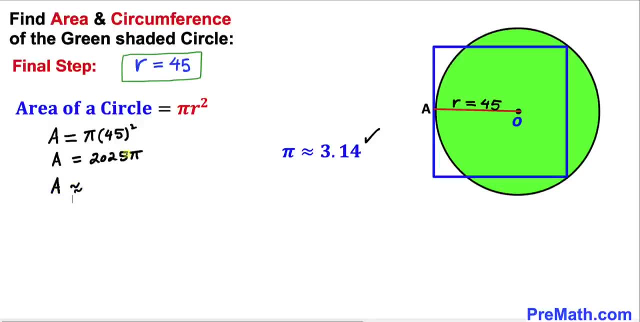 going to be approximately equals to 63, 61.7 square units. and now let's go ahead and calculate the circumference of this green circle. and here's the circumference of a circle formula, which is equal to 2 pi r. let's go ahead and fill in the blanks, so our circumference c is going to be 2 pi times our. 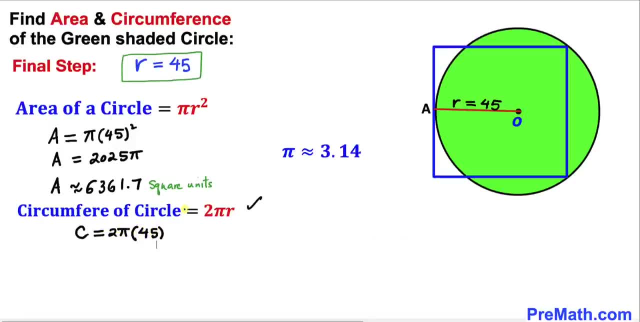 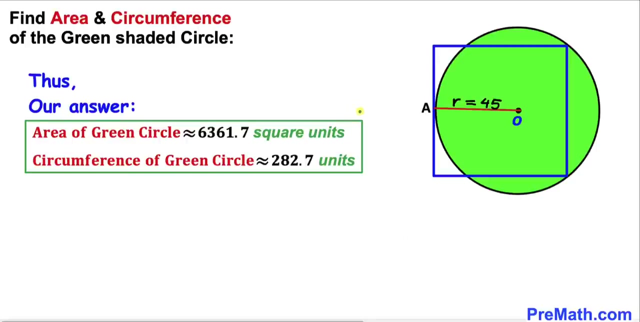 radius is 45 units. therefore, our circumference is going to be 90 pi units, but we know our pi value is approximately equal to 3.14, so we are going to plug it in. so our circumference is approximately equal to 282.7 units. And here are the area and the circumference of this green circle. 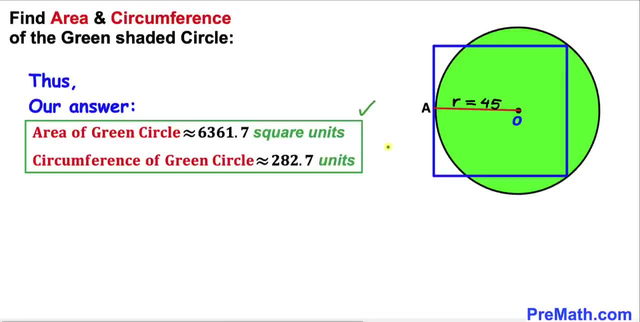 Thanks for watching and please don't forget to subscribe to my channel for more exciting videos. Bye.